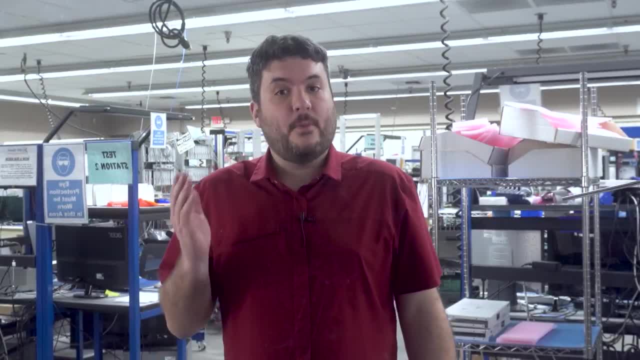 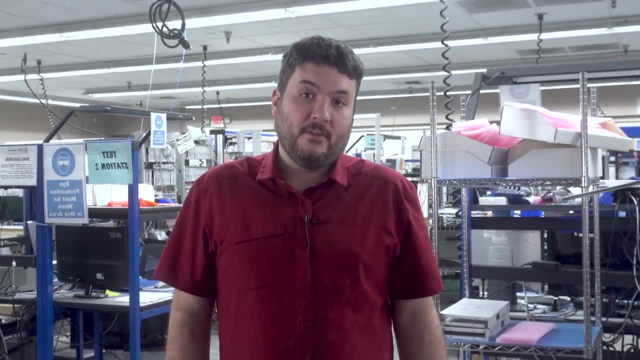 The exchange of information in SNMP protocol can be done via polling or via traps. If you manage a network that operates on SNMP, you need to understand the difference between these two methods. I'm going to show you the difference between SNMP polling and SNMP traps. 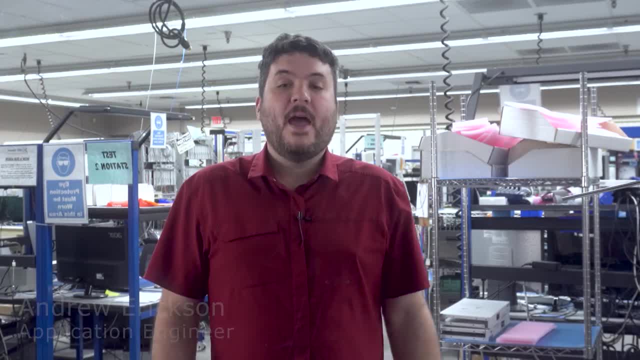 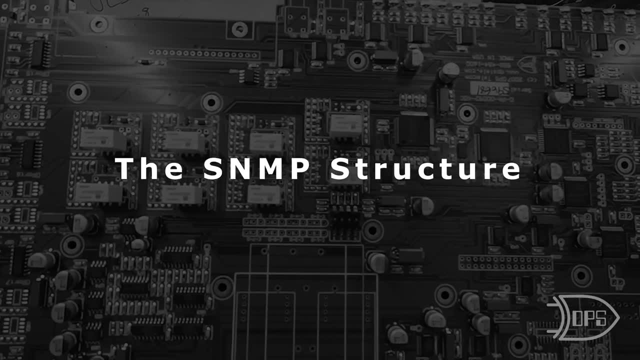 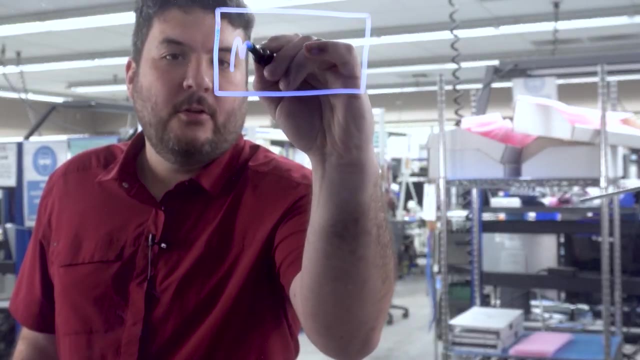 Hi, I'm Andrew from DPS, Welcome back. SNMP is a standard communications protocol in network monitoring systems. SNMP is based on the manager and agent model. You'll have a single manager. This is your central hub of information, where all sorts of data gets collected. 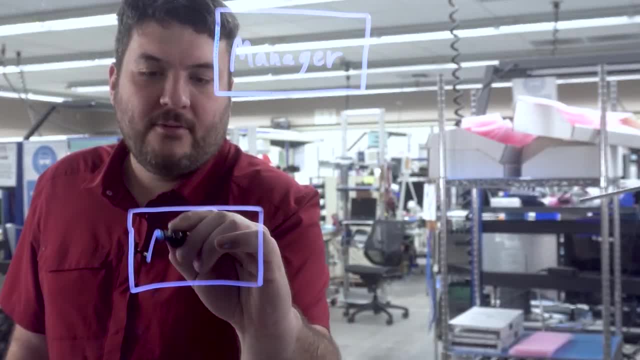 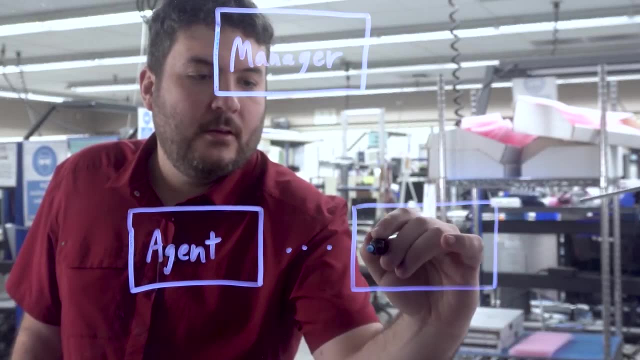 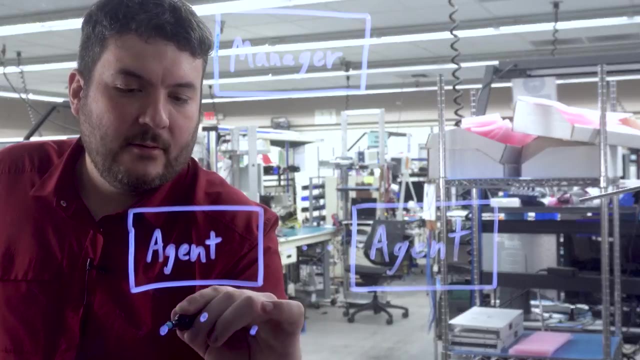 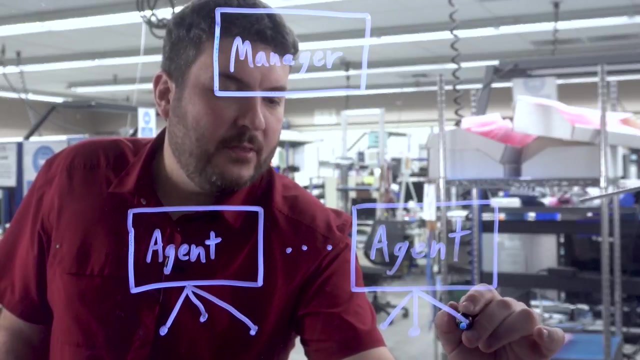 And then at various remote locations you'll have SNMP agents, And we can have many. I'm just going to draw two with an ellipsis here. The job of an agent is to collect various pieces of information from out at their location. They might also report information they just get from within themselves like little system alarms. 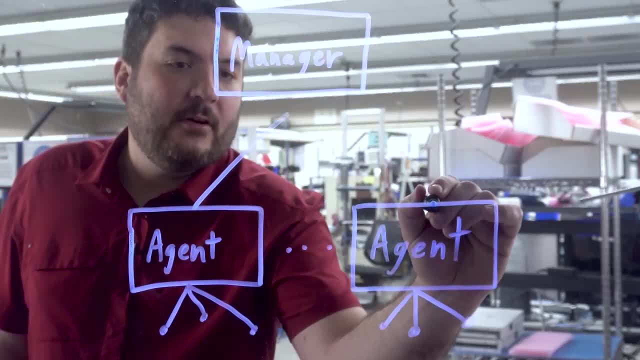 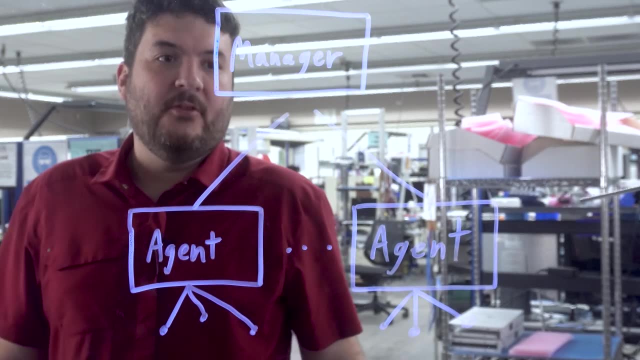 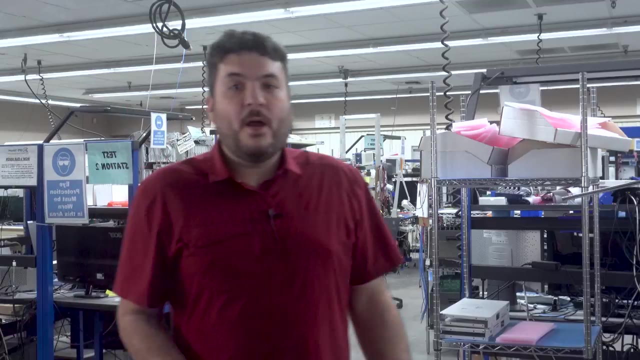 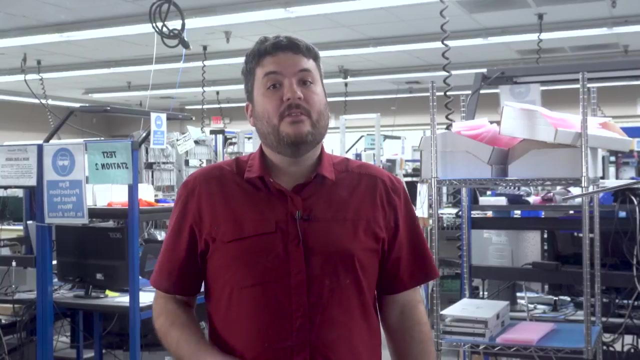 And the job is to communicate back to the manager. That way, you can view all the information right there in your central information hub. The precise way that your SNMP manager and your agents talk to each other is traditionally via asynchronous SNMP trap messages, But some systems may use polled messaging instead. 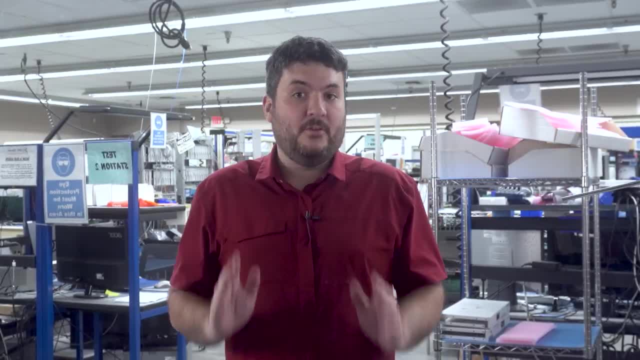 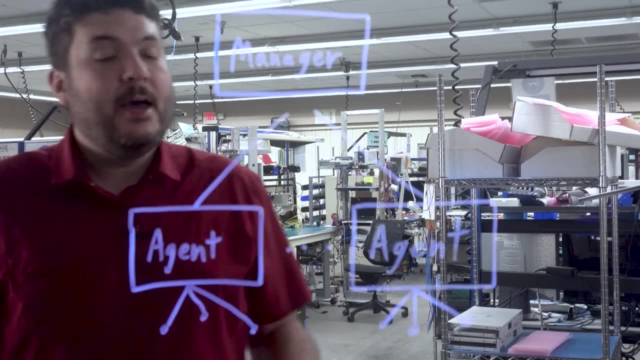 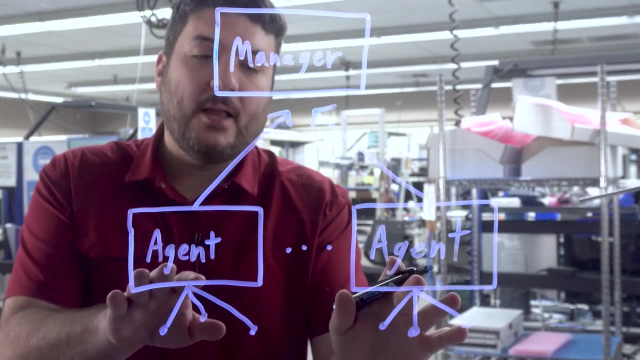 Let's look at what these two methods are and what makes them different from each other. Traditionally, SNMP is asynchronous. This means that your agents are going to send SNMP trap messages whenever something notable happens, But the manager is not going to be asking for information on any kind of predictable schedule. 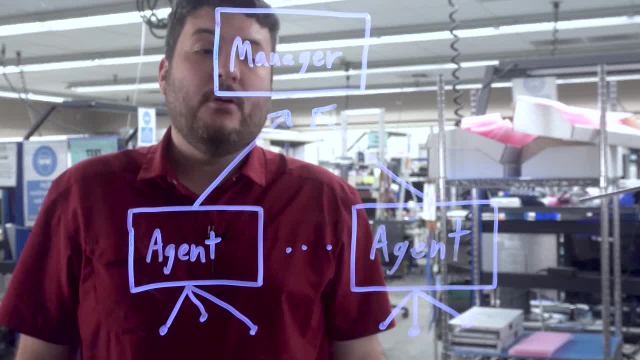 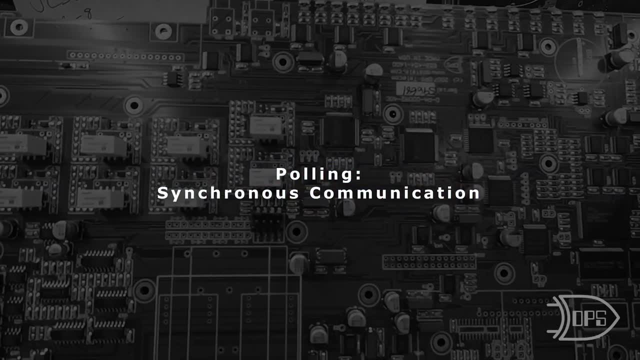 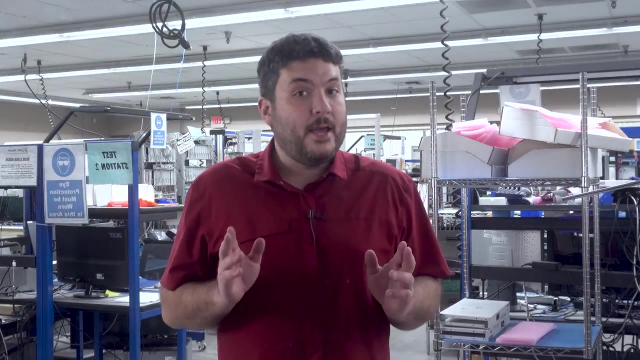 So if you get silence from an agent, you don't know if that means everything's okay or it could mean one of these agents is offline and you have no way of knowing. This limitation is addressed in some other protocols And, more recently, some SNMP devices also use a polled method instead of sending traps.